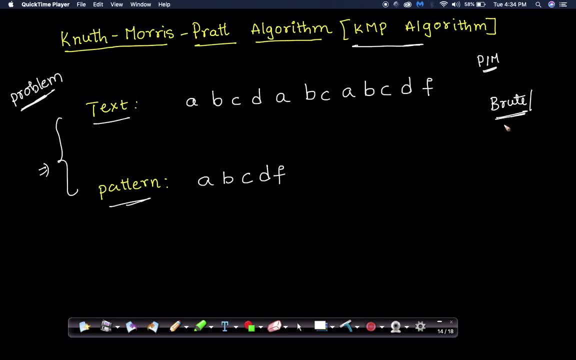 have discussed one of the string matching algorithm called a navi based approach. okay, what we have done in this navi based approach every time we are going to compare each and every character, right? what I am telling you here is: let's suppose here my given pattern containing how many number of 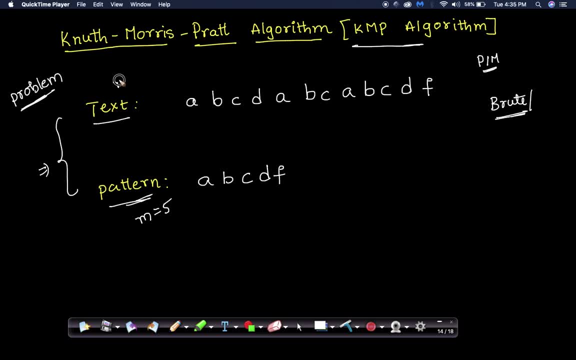 character, five, number of character and the given string containing how many? number of character: three, six, nine, twelve, four, number of characters. okay, according to the brute brute force approach, what we will do, we are going to compare. I'm going to take this pattern. okay, let's start from the starting index of the string. okay, that, 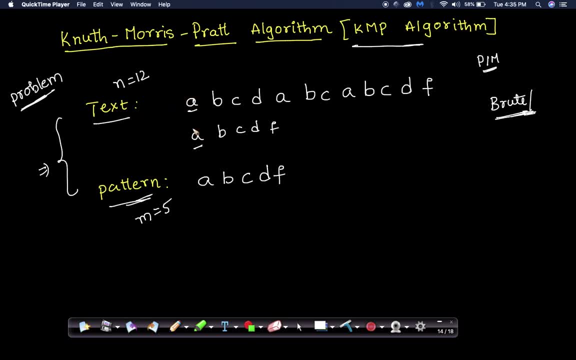 is the given text. okay, now I am going to compare and starting characters of these two. okay, that is a with a- yes is matched. then I will go to the next character, that is B with B yes is match. next I will go with the next character, that is: 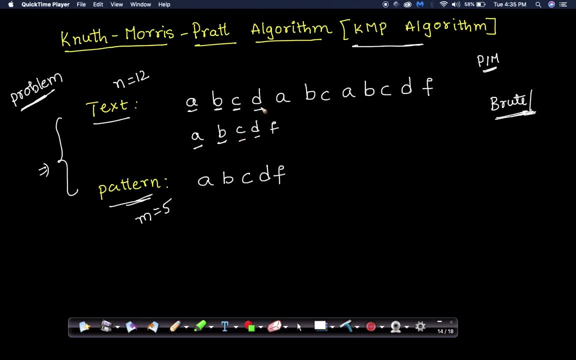 C and C. yes, it's match. then I will go to the next character, that is, D and D. yes, it's match. then last character, A and F. we got a mismatch here. okay, according to the brute force approach, what will we do again? we are going to start from this index, right? 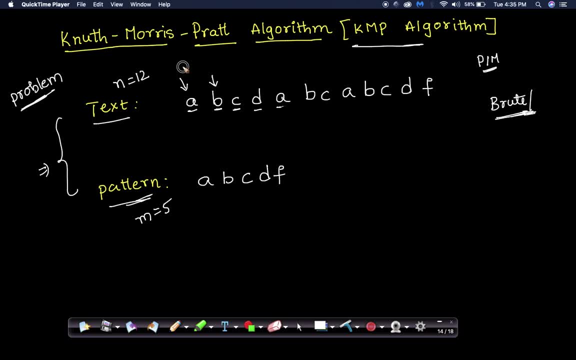 okay, initially. okay, let's take this pointer. I am going to start. take that one pointer, name it as I and I am going to name it as J here. okay, initially, what we have done here is: first we are going to start from zeroth index. okay, I is. 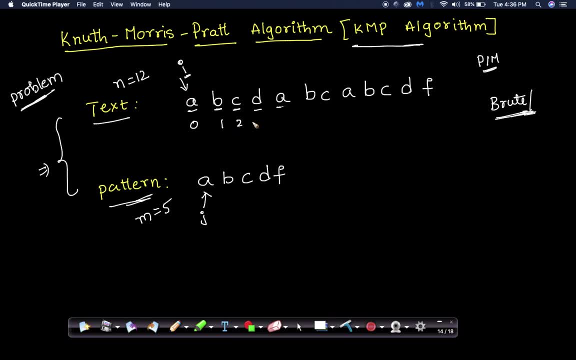 starting from zeroth index. okay, zero one, two, three, four, five, six, seven, eight, nine, ten and eleven. okay, these are my indices of this string. okay, then, I am going to start the indices of J from zero. okay, this is zero one, two, three and four. okay, my I is at the zeroth index and J is at the zeroth index. now I am. 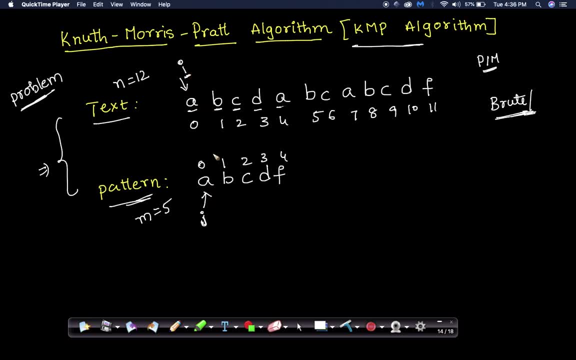 comparing I and J. okay, what is the value present in the I and J are A and A. yes, it's match. then I will increment the value of I and as well as I am going to increment the value of J as well. okay, right now my J is pointing to the first. 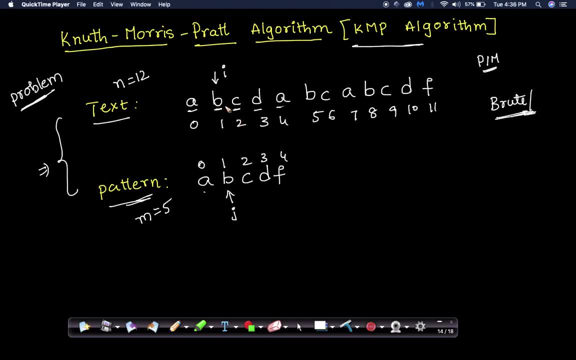 index, and I is pointing to the first index of this text. okay, then I will compare and the value presented I and J indices, that is, B and B. yes, it's match. then I will going to increment the value of I and as well as increment the value. 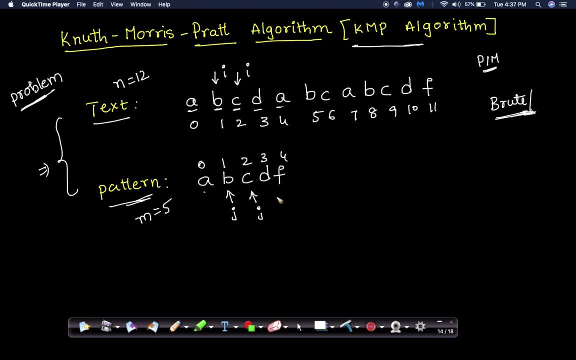 of J. okay, then I will compare C and C. yes, it's match, then I will go to increment the value of J, as well as B and B. yes, it's match, then I will go to increment the value of J as well as increment the value of J. okay, then I will compare C and C. yes, it's match, then I will go to increment the value of J as well as increment the value of J. okay, then I will compare C and C. yes, it's match, then I will go to increment the value of J as well as. 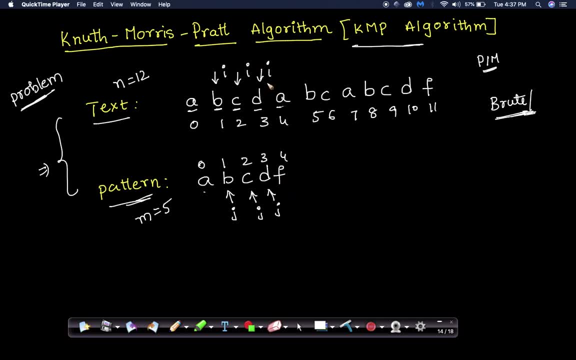 increment the value of I, then I will compare the value present at the indices of I and J, in this case D and D. yes, it's match. then what we have to do? we have to increment the value of I and as well as increment the value of J in. 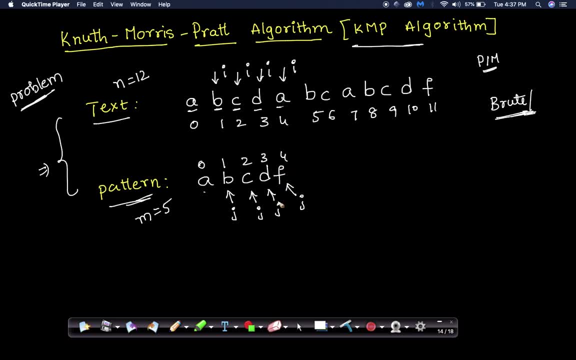 this case there is a mismatch, that is A and F. okay then, what will we do? according to the brute force approach? again, we will go back to the previous again. I am going to start from the indices one. okay, we will start what we have done in the initial step. we started. 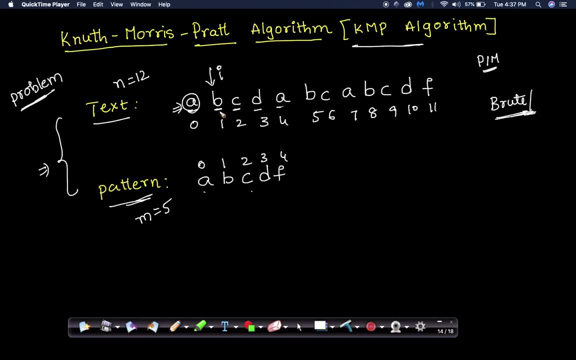 from the previous two indices. okay, what we have done in the initial step we started from from the first character. then I am going to start from the second character. then again I will go back and I am going to initialize my j with 0. then I will repeat the same step. right, that is what we. 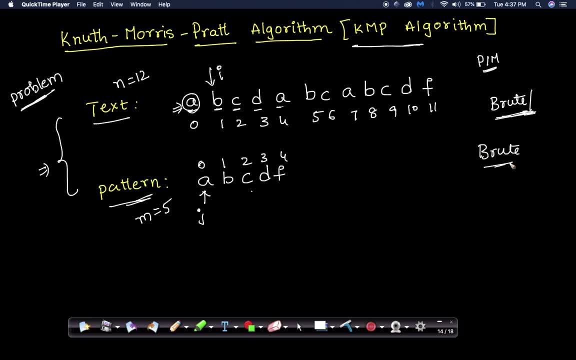 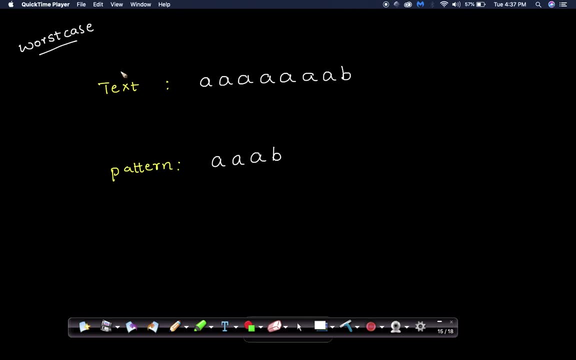 have done in the brute force approach. right, and what is the time? complexity of this approach, this order of n into m? right, okay, why? let's take this worst case. okay, let's take another example so that we can understand it. why it's order of n into m? okay, let's suppose this is my given text. 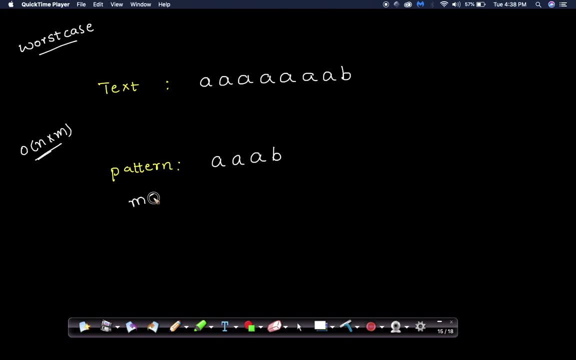 and this is my pattern. how many number of characters present in this pattern? that is, four number of characters, and in the text, how many number of character? that is, n is equal to 3, 6 and 8. okay, and according to the brute force approach, what will we do? this is my indices of. 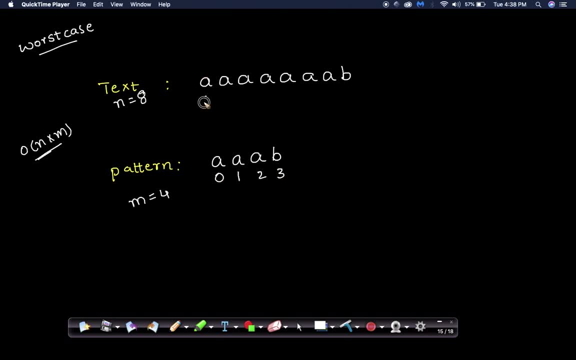 the pattern 0, 1, 2 and 3. these are the indices 0, 1, 2, 3, 4, 5, 6 and 7. okay, and I am going to take two pointers, that is, i and j. okay, what we have to do first I am going to compare the values present at the indices i and j in this. 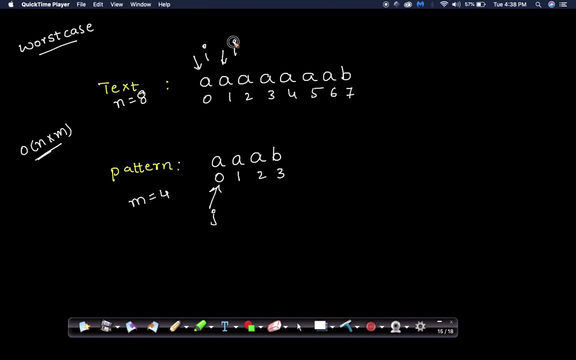 case a and s? s is match, then what we have to do, we have to increment the value of i and j parallelly. okay, and a and a? s is match, then I will increment the value of i and as well as increment the value of j by 1. okay, right now I am at the indices 2 and the value presented, both the patterns. 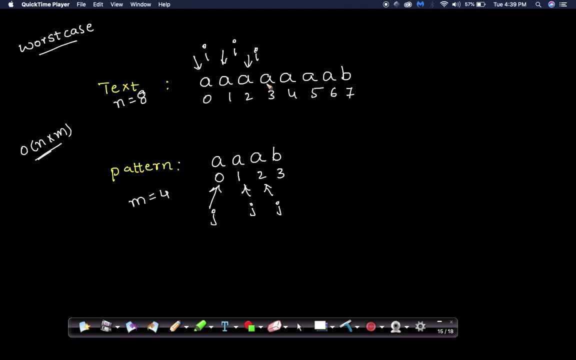 are, our strings are same characters, that is, a and a, then I will going to increment the value of i and s increment the value of j. okay, in this case there is a mismatch. okay, then, what we have to do again, my i will come to the first point, that is, the first indices, and j will point into the 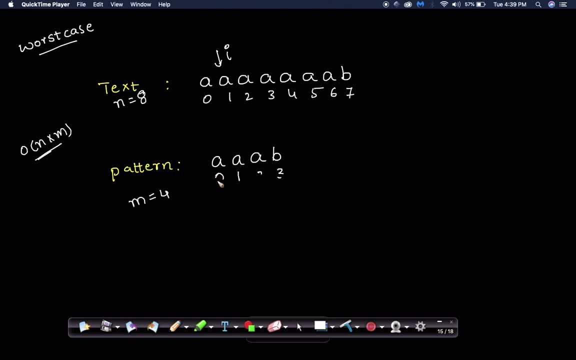 zeroth in this. okay, what is the drawback here? we are comparing again and again. right, we have seen there are three a's present and there are three a's still. we are going back to the previous indices. okay, we have traversed three number of characters. we have seen some number of characters matched. 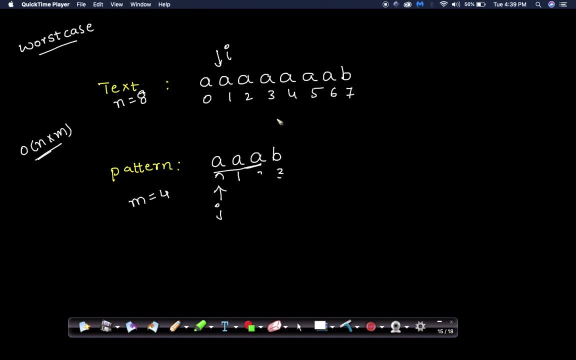 with the against the previous indices. okay, we have seen some number of characters matched with the actual text, but there is a mismatch of single character. we are going back to the again, the starting position. that is the main drawback of main drawback of this brute force approach, right? 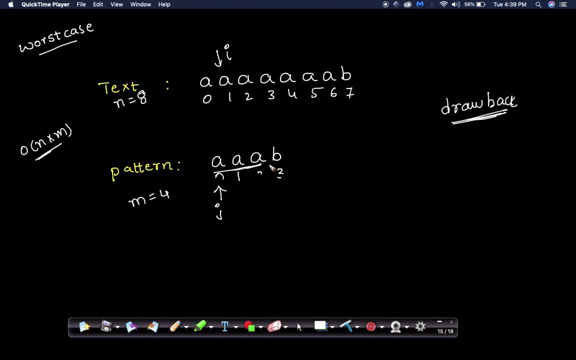 okay. that is why, in the worst case number of comparison it will take, in the worst case, for each and every character we are going to compare with m time there are n number of characters present in the text, then total time complexity of this brute force approach is order of n into m. 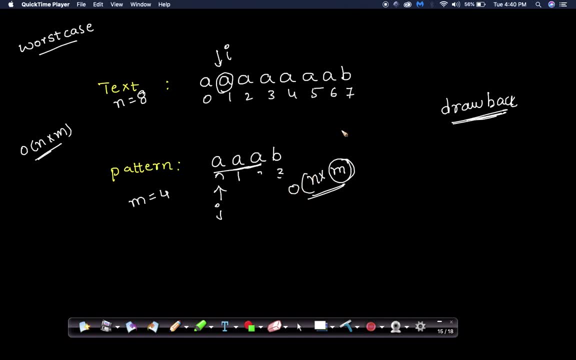 okay, then, how to overcome this. okay, that is why- and these three scientists proposed an algorithm. okay, based on this pattern, because we have seen some of the characters already visited and we have seen that appeared in the given text. but instead of repeating again and again, okay, they have. 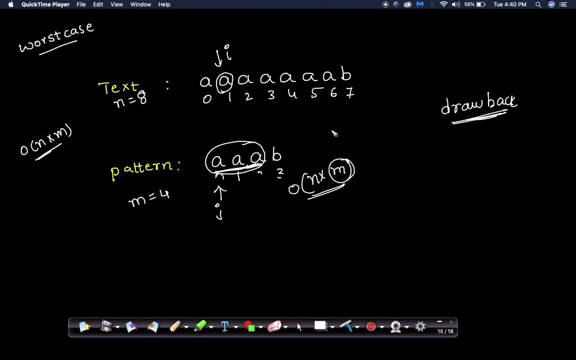 proposed one algorithm. okay, that is called a kmp algorithm. okay, let's understand the basic terminology of this kmp algorithm first. later on we will see what exactly they have proposed it. okay, let's suppose this is my given pattern. okay then, and first understanding this kmp algorithm. first we should understand the concepts of prefix and suffix. 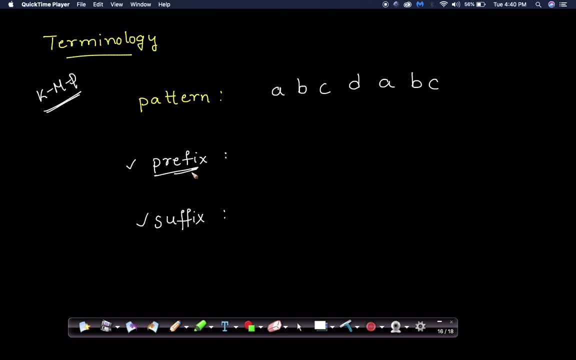 okay, and we have already known about the prefix. right prefix is nothing, but these are the subset of string present in a given input string. we'll start from the left side of the pattern. okay, what i'm telling you here is the free, and in this example, A is one of the. 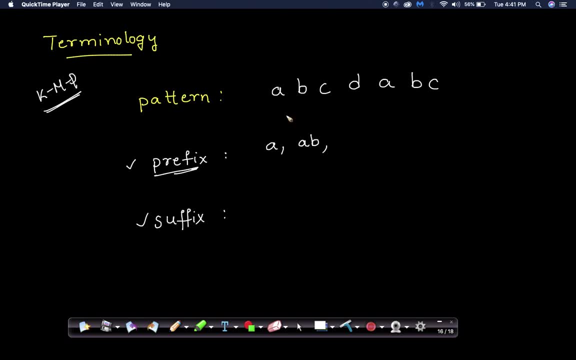 prefix and AB is also the prefix, then so on. as i mentioned, you can find more Taiwanese patterns. a prefix. I'm going to start from this: left side, right, and ABC is also a prefix and ABCD is also a prefix. okay, this is my given pattern. it's not a text. 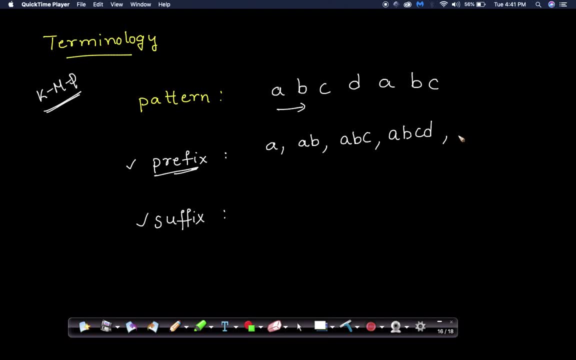 I'm just taking as a pattern here: okay, and ABCDA is also one of the prefix. okay, and so on. okay, for this given string. these are the possible prefixes, right? and similarly, what about the suffix? suffix will start from the right side of the string. okay, that means C is one of the prefixes and BC is also one. 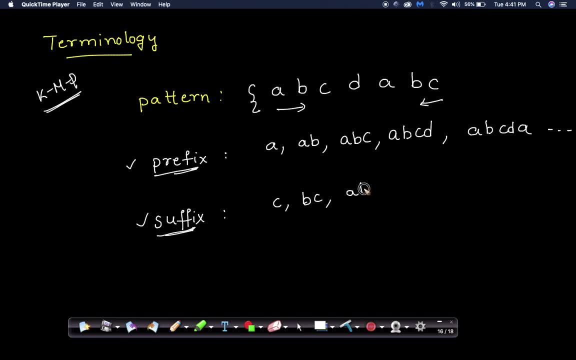 of this suffix, and ABC is one of the suffix, and DA, BC is one of the suffix, right and so on. okay, if you can carefully notice here, is there any prefix which is same as suffix? okay, A, I'm going to compare a. is present in the suffix or not? in this case, no, and AB is. 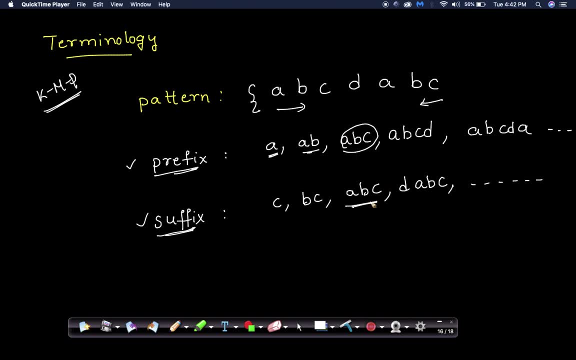 present no and ABC. Yes, there is a match. Okay, That means same string. Okay, Here that same prefix is appeared in the suffix- That means my, some of the characters present in this beginning of the string, and is also appeared in the later part of the string. Okay, That is the main observation. 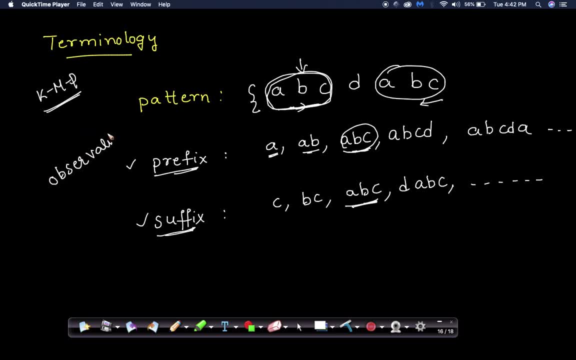 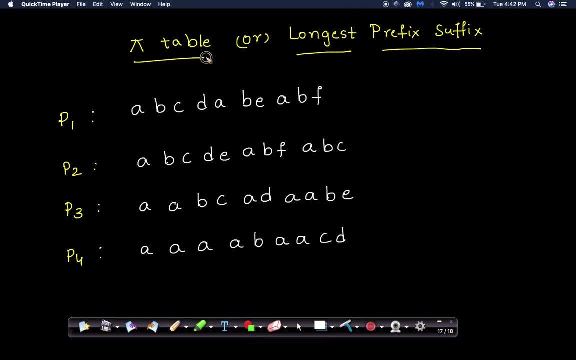 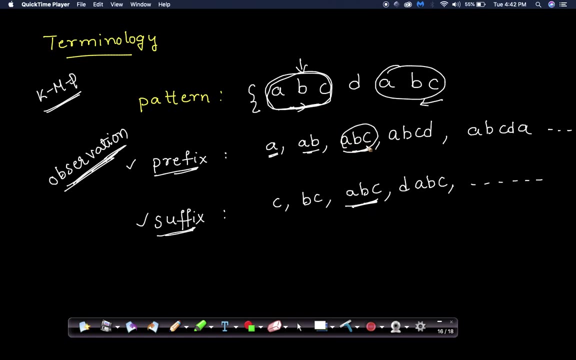 done by the, these three scientists, Okay, And based on that, they have designed an algorithm. Okay, And for that, first, they have to prepare a table called a pi table. Okay, And based on this, this concept, what we have observed here is there is a common prefix and suffix are there in the 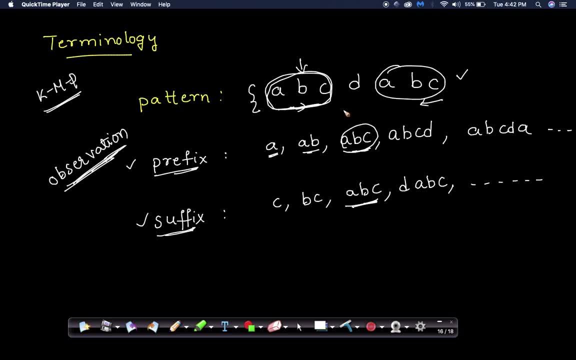 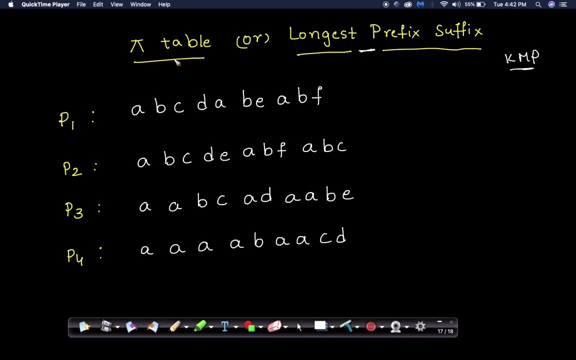 given input string. Okay, Then how can we maintain a table based on that? once you maintain this table, okay, and construct this KMP algorithm is very, very simple. Okay, Let us understand how to construct this pi table For better understanding. instead of you know, there is a terminology of prefix and. 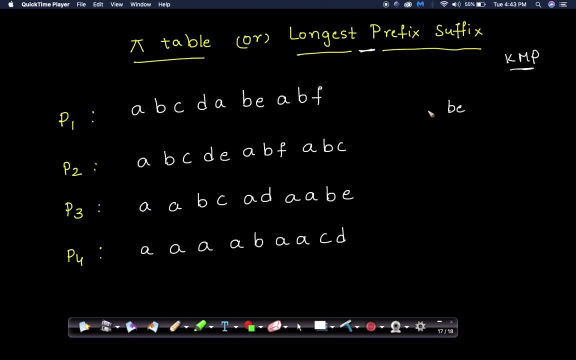 suffix. instead of that, I am just maintaining beginning of. if there is any beginning of, the characters is present. Okay, Beginning string is present in the later on any other string? Okay, In the given input string. Okay, Then I am going to represent it in a pi table. Okay, I will. 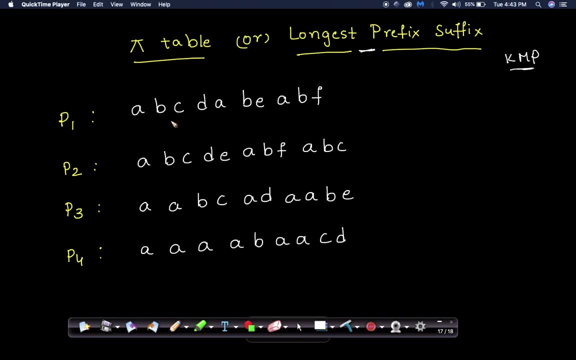 show you here how can we construct a pi table here. Okay, Now what I am going to do here is first, I am going to start from a. Okay, And is there any a present later on in this string or not? I am going to check it. Yes, A is present and a is one. 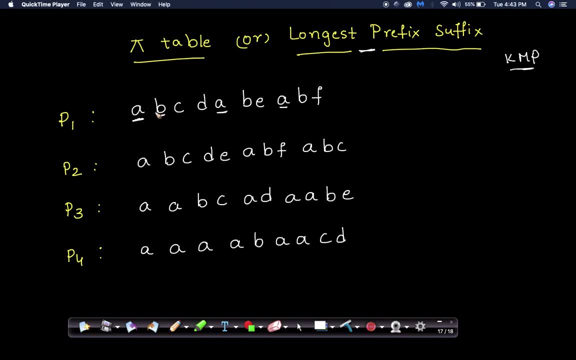 A is present and b is also present, right and adjacent to each other. These two are adjacent to each other. Yes, A and b are present here and a and b are present here. Okay, Then, what I am going to do here is: I am going to represent the indices. Okay, I am going to take the indices value. here is: 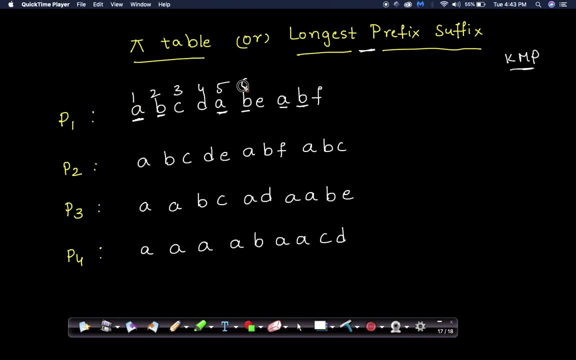 1,, 2,, 3,, 4,, 5,, 6,, 7,, 8,, 9 and 10.. Okay, Then, what I am going to do here is I am going to put here for one time occurring, and I am going to put it as the indices of that. 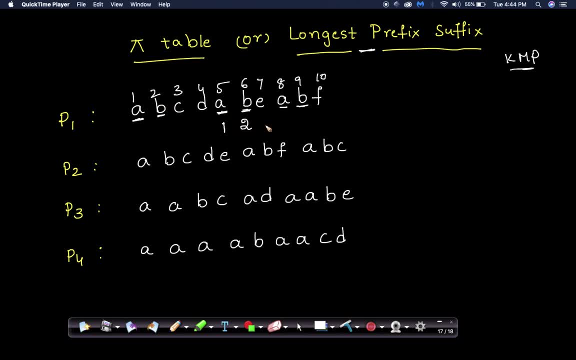 here. Okay, And for, similarly, for b, I am going to put it as 2.. And what about this case? that is, 1 and 2 and remaining all? I am going to put it as 0.. Okay, For better understanding, I have taken this: 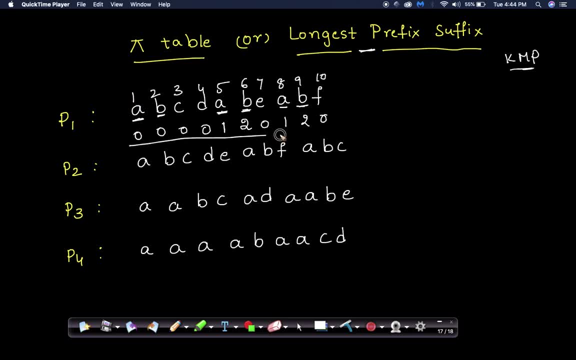 you know, indices start from 1. here I have constructed a prefix or LPS table. Okay, LPS is nothing but longest prefix suffix table. Okay, I hope you understand this right. What is prefix suffix table? that is the same substring is appearing later on in the same string. Okay, 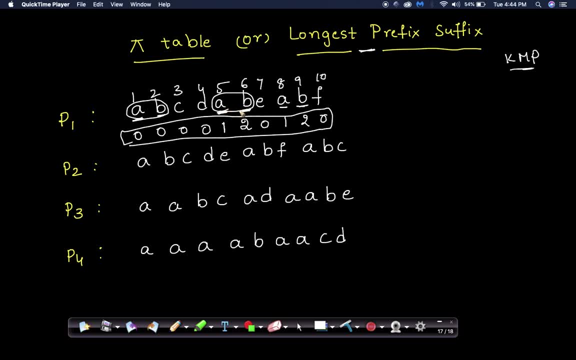 If you carefully notice this thing, a b is present here itself and a? b is also appeared one more time. Okay, For that reason, I am going to maintain one table here. We call it as the table, as either pi table or a longest prefix suffix table. Okay, Similarly, let us take this example. Okay, Let us. 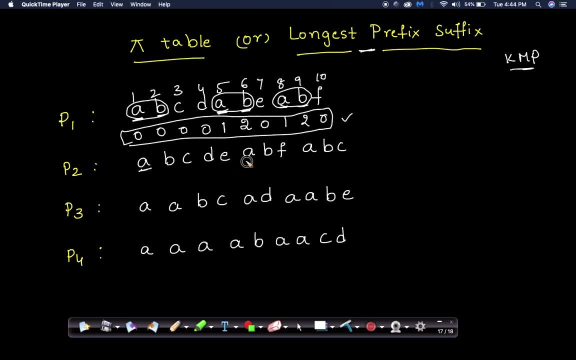 start from a. a is appeared anywhere in the string. Yes, a is appeared here. a is appeared here, Okay. Similarly, b is appeared. Yes, b is appeared. a b is appeared. a b is appeared Okay. And a b- c is. 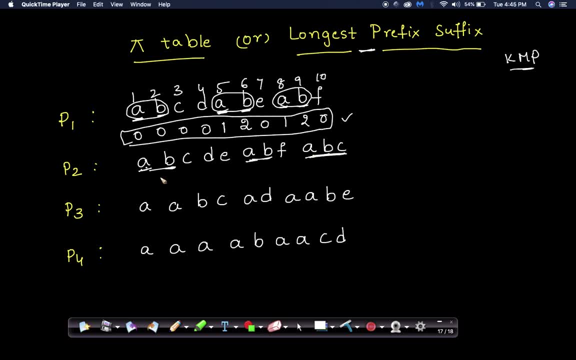 here. Yes, It is there Right In the last string is appeared. Okay, For that. first. I am going to maintain here: 1. Okay, Because of starting indices is 1 and b, starting indices is 2 and similarly a, 1, 2 and 3.. Okay, Remaining all characters, I am going to put it as 0.. This is my prefix. 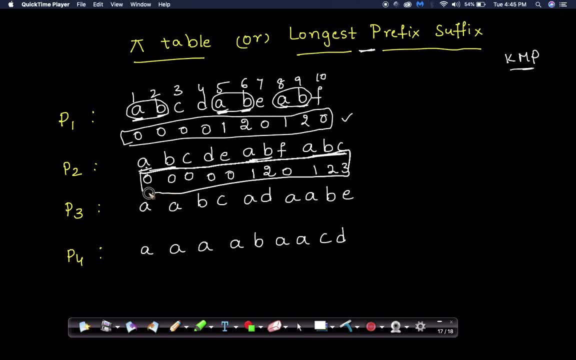 longest prefix suffix table. I hope you understand this right. Let us take this example. Okay, Let us start from a. Okay, a is present anywhere else in the string. Yes, It is near to here. Right, Then I am going to put it: 1 here and similarly, 1 is present here and 1 is here, and. 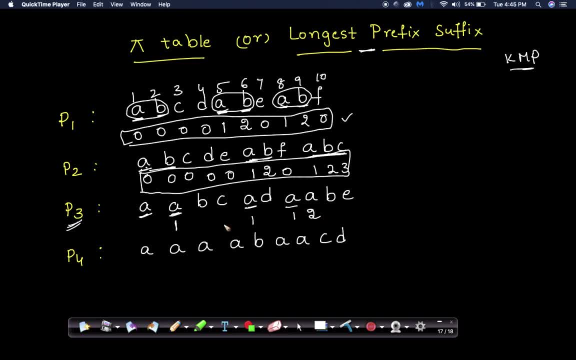 1 is one more. 1 is present adjacent to each other, Then I am going to put it as 2.. Okay, I hope you understand this right. This is 1 and 2, and 2 is also containing the a. I am going to put it as 2. 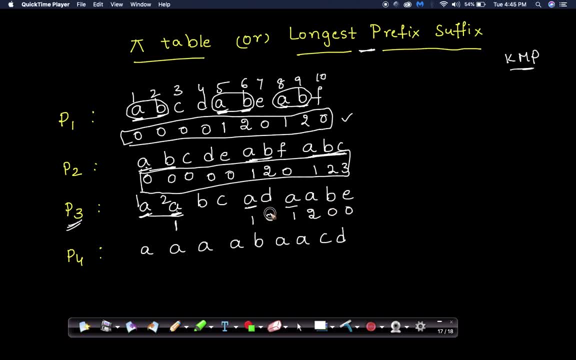 here and remaining all other characters, I am going to put it as 0.. Okay, I hope you understand this right. It is a very, very simple to construct a prefix suffix table that is longest prefix suffix table. It is trivial to solve the KMP algorithm. Okay, This is the main logic and the main. 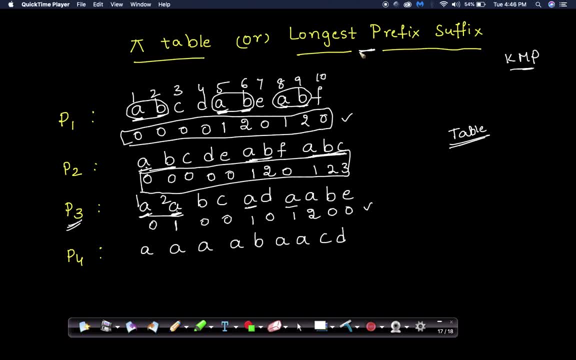 important thing for this KMP algorithm is construct a longest prefix suffix table. Okay, Let us take this one more example. Okay. After that we will go back to our actual algorithm proposed by the KMP algorithm. How can we find that pattern? Okay, And what about this one? Okay, How can we? 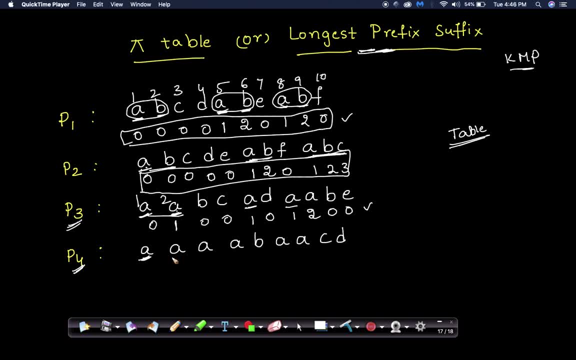 construct this table. That is first. I will start from a. a is appeared here, Then I am going to. one more a is appeared, I am going to put it as 2, and one more a is present. I am going to put it as: 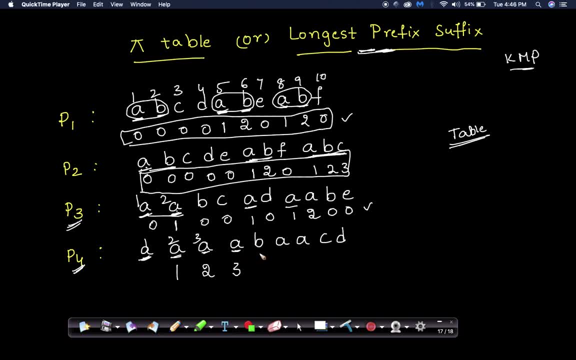 3, because 1, 2, 3 adjacent to each other. Okay, Then I am going to put it as 1 and 2 and remaining all are zeros. Okay, This is my. this is the way of constructing a longest common prefix prefix. 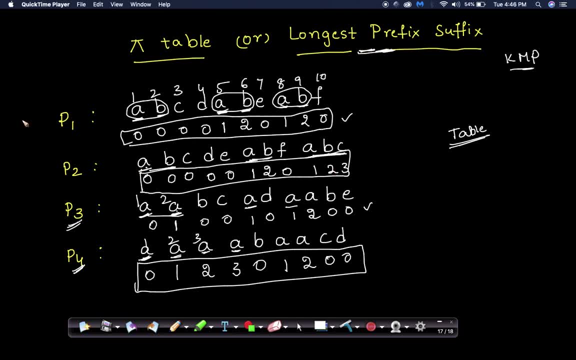 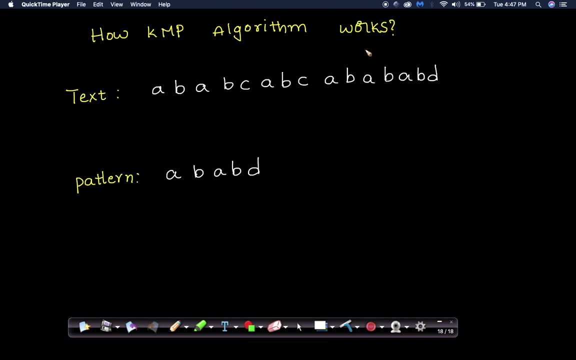 longest prefix suffix table or a pi table. I hope you understand this right With this many number of example. I hope you understand this: how to construct a pi table. Now we will go back to our actual problem: Actual algorithm proposed by the KMP algorithm. Okay, Now we will discuss how KMP algorithm works. 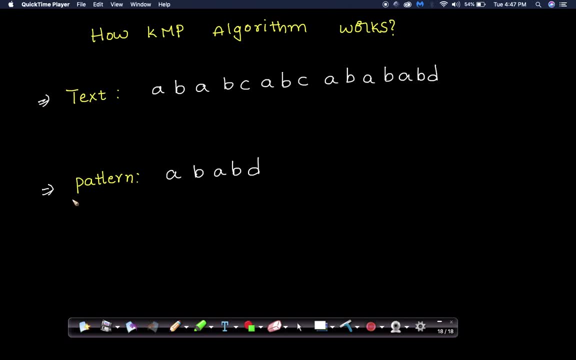 Okay, Let us suppose this is my given text and this is my pattern, and how many characters are present in this pattern? That is 5. number of characters, and how many characters are present in this text, That is 3, 6, 9, 12 and 15.. 15 characters are present in the given input string. 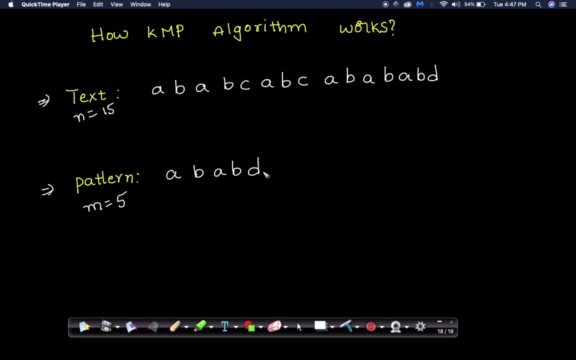 Then our main task is to find that given Pattern is present in the text or not, using the KMP algorithm. Okay, And the initial step. what we have to do? we have to construct a pi table. Okay, How to construct the pi table from the pattern. 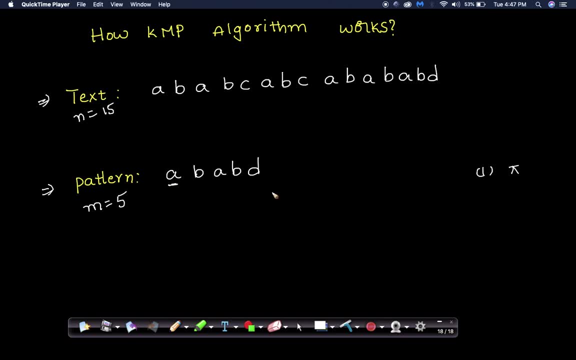 First I am going to check from: a is anywhere present in the string or not? Yes, it is present and I am going to put it as 1 and b is present. Yes, I am going to put it as 2 and as well as any. 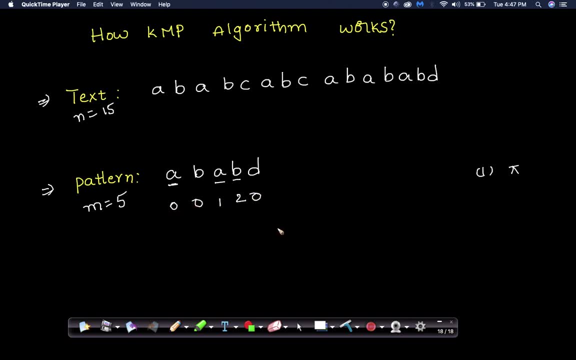 other characters. No, right, I am going to put remaining characters 0.. Okay, Let us draw this as a table. Okay, And I am going to put it as 1 and b is present. Yes, I am going to put it as 2 and. 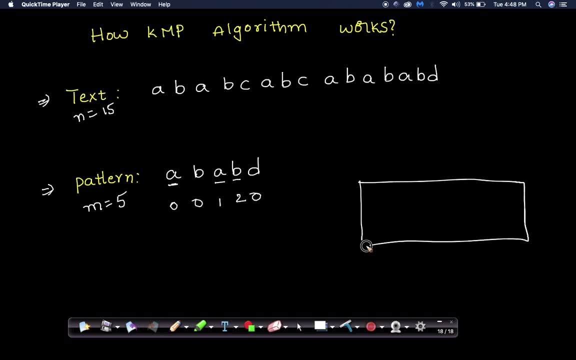 as well as any other characters. Okay, I am going to put it as: 1 and b is present. Yes, I am going to construct this table. This is my pi table, Okay, And how many characters are present? 5 characters are present in this given pattern And what are the characters? That is, a, b, a, b and d. Okay, Right, 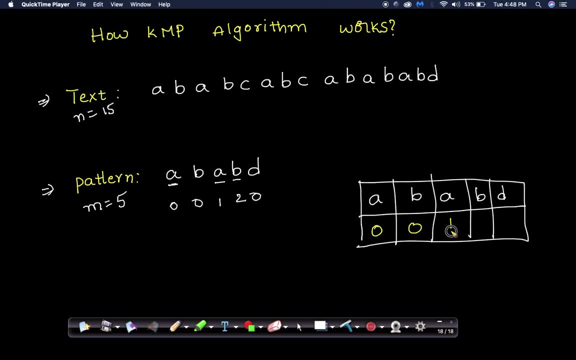 And what are the values, That is, 0, 0, 1, 2 and 0.. Okay, Here these are nothing but indices 1 and 2.. That means we have seen this. a, b is appeared again. Okay, We have to remembering the things. 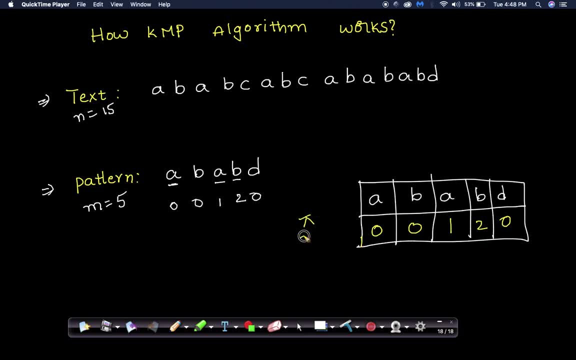 we have constructed table here. we call this table as pi table. right now, let's see how kmp algorithm works. okay, then i'm going to put it as indices here: 1, 2, 3, 4, 5, okay, and i'm going to start from 0. i'm going to take one more indices, that is 0. i'm going to take- uh, i'm going to point. 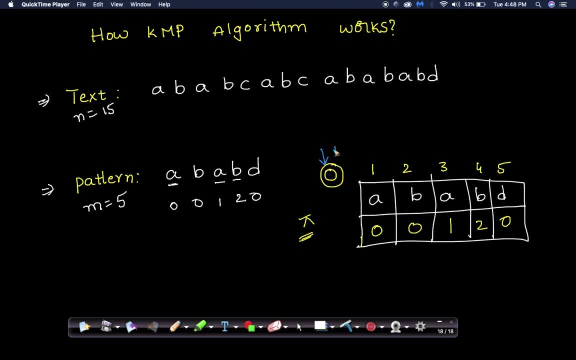 another. i'm going to take another variable called a j, which start from 0 here. okay, for better understanding, you can also start from here. for better understanding, i'm going to start from 0 here. okay, then, as well, as i'm going to take one more pointer, i here. okay, then, what i'm going to. 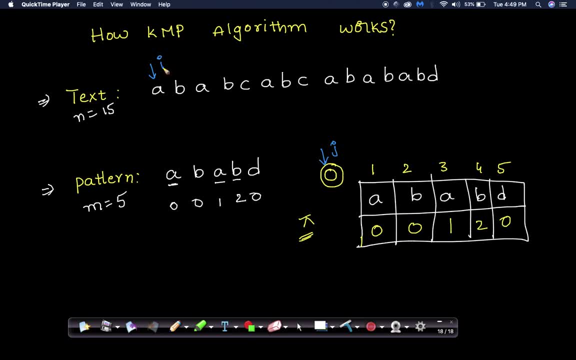 do here is: i'm going to compare my i i'th index value, that is a and j, plus 1 index value. that is a right, and if there is a match, then what we have to do i'm going to increment the value of i, okay. 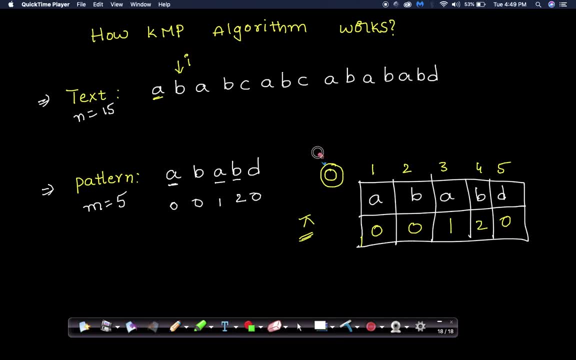 then i move the pointer of i by one index and similarly i'm going to move the pointer of j by one index. right now, my j is pointing to the first index and similarly, my i is pointing to the first index. let's, let's name this indices value. okay, this is my first index, i'm just for. 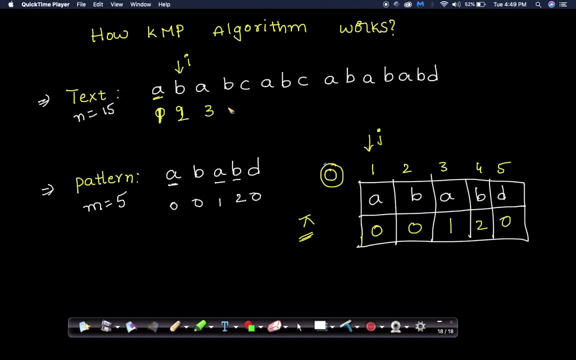 understanding purpose. i have just representing like this: 1, 2, 3, 4, 5, 6, 7, 8, 9, 10, 11, 12, 13, 14 and 15. okay, right now i'm at the second index. okay, that is the second characters of the given input. 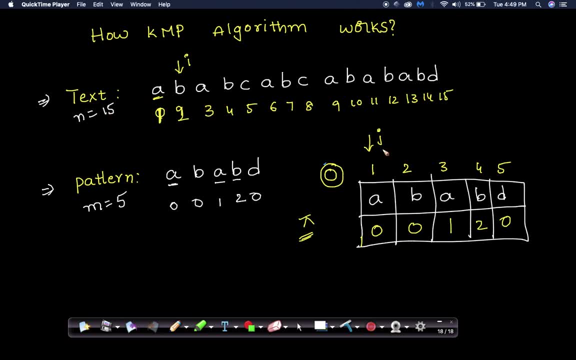 string. then what do i do? i'm going to take one index. i'm going to take one index. i'm going to have to do, i'm going to check this: j plus 1 index value. that is what is the value. that is b. i'm going to compare the ith index value. that is b. yes, it's a match. then what i'm going to. 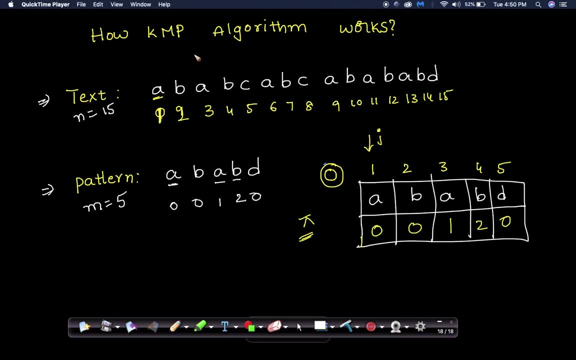 do here is: i'm just going to increment the value of i by 1. right now, my i is pointing to the third index and j is pointing to the second index. right and again, i will repeat the same step. then how will we compare? that is, ith value, that is a, and j plus one index value, that is a. 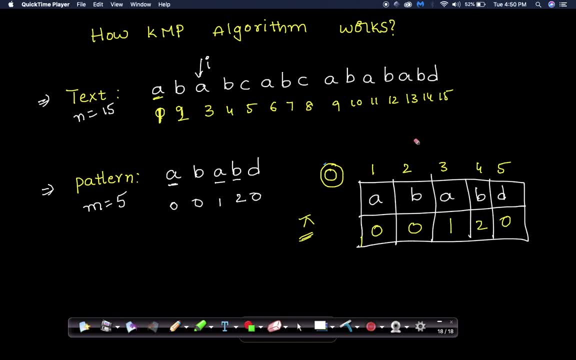 yes, it's a match. then what we have to do? we have to increment the i and j one pointer ahead. my j is pointing to the third index and similarly, my i is pointing to the fourth index, right now. then again, i will going to compare j plus one index value, that is b, and ith value, that is the value. 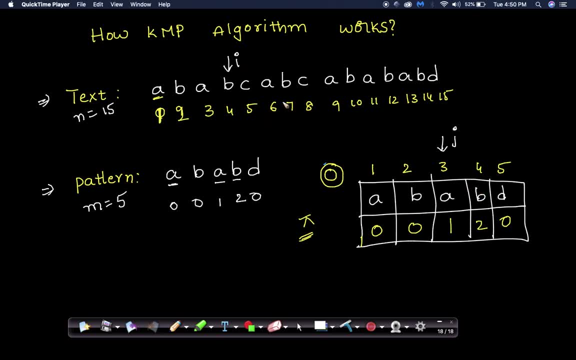 present at the ith index is b? s. there is a match. then what we have to do? we have to increment the of i by 1. okay, right now i am at the fifth index. okay, then i am going to increment the value of j by 1 index. okay, right now i am at the fourth index of the j. okay, then, what we have to do, again, i will. 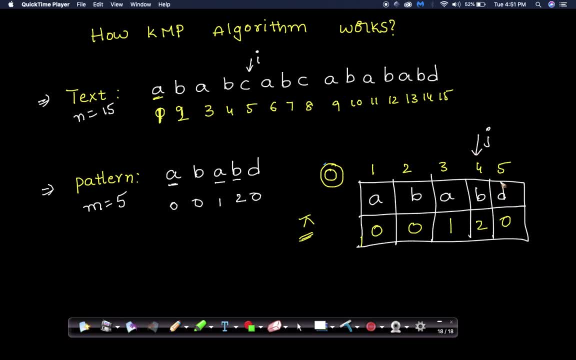 repeat the same step. the value present at the j plus j plus 1 index, that is d. i'm going to compare with the ith index, that is, ith index value is c in the given input string. okay, there is a mismatch. then what we have to do instead of in the? 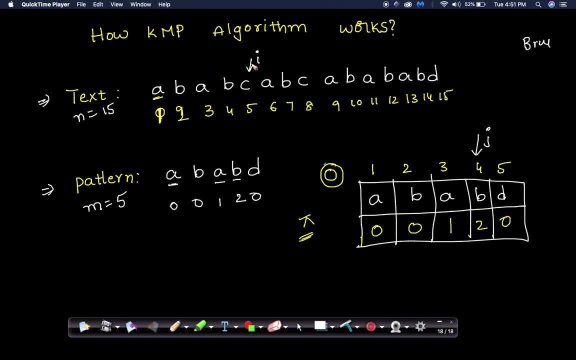 brute fun approach. what we have done again this: we are backtracking this i to this first index. right, that is the second index. we are going back again and we are going to start from here. that is the main drawback of the brute force approach. instead of doing that, what i am going to do here is: i am 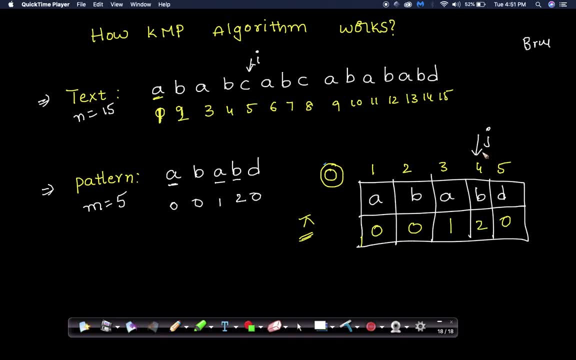 just moving my j from here. i want to move my j to this position. that is second position, because i have seen a. b is already appeared in the given input string, as well as the pattern. that is the reason i, instead of moving my i back to the previous position. i am just in the you know. 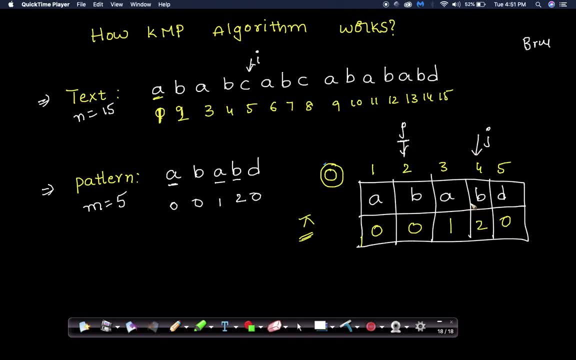 going back, my j position. that means we have seen that a, b is appeared one time already in the given input string. okay now, right now, my j, at pointing to the second index. okay, then again, i will repeat the same step. okay then, what is the value? j plus one? value is a and ith index value is c. yes, there. 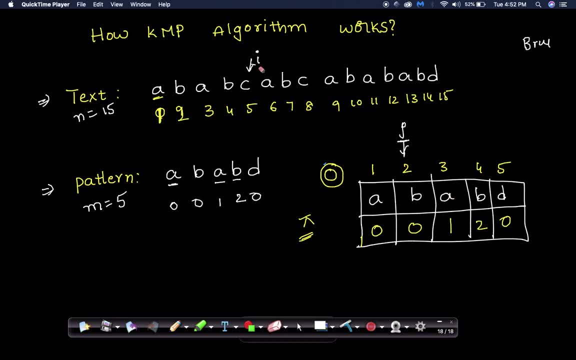 is a, again there is a mismatch, then what we have to do, instead of moving my j to this position, i am just moving my j to this position. i am just moving my j to this position. i am just moving my j to this position. that is the zeroth position. okay, that is the main. 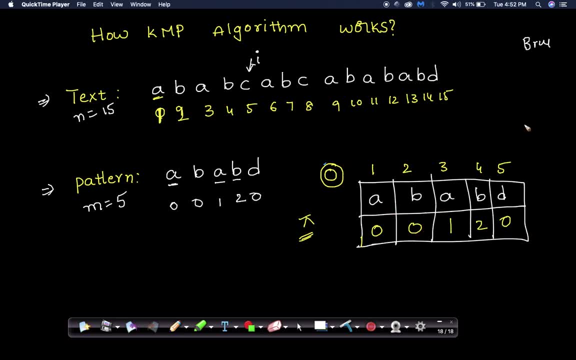 advantage of constructing a longest common, longest prefix suffix table or a pi table right, instead of moving my i back to here, i am just moving my i j here. okay, right now my j is pointing to the zeroth index. okay, then again, i will going to compare my j plus one index with the ith value. 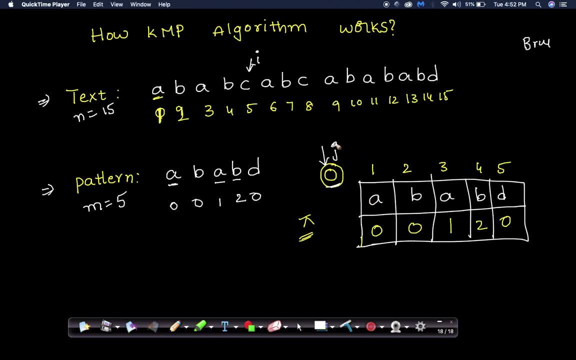 in this case, yes, there is a again, there is a mismatch. my j is pointing to the zeroth index. pointing to the zeroth index, that means i am at the starting. then again, then what i will do here is i'm going to, i'm going to increment the value of i by one. okay, then i'm going to compare it. 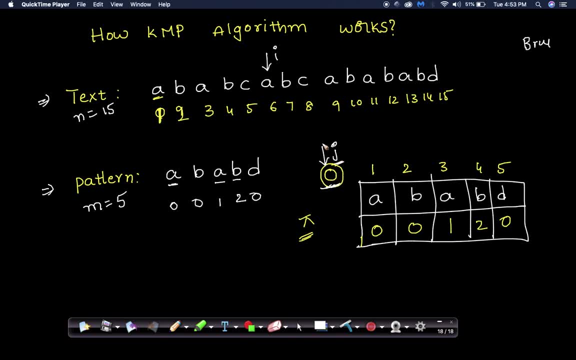 again. okay, that means again, i am at the starting position. there is a mismatch, then i'm going to increment the value of i by one. okay, then again i will repeat the same step. okay, what we have to do? we have to compare the ith index value, that is, a and j, plus one index value is a. yes, it's a. 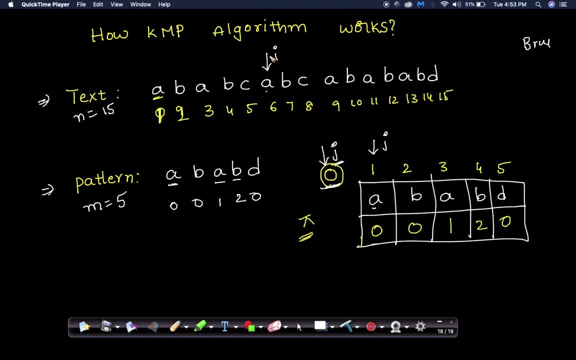 mismatch. then then increment the value of j by one and increment the value of i by one. okay, then j plus one. value is b and ith value is b. yes, it's a match. then i'm going to increment the value of j by one and increment the value of i by one. okay, and j plus one. value is a and ith value is c. that 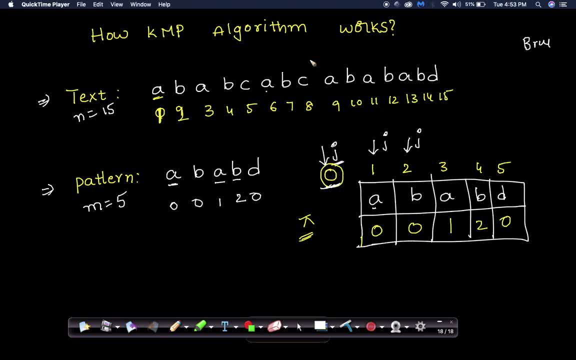 means there is a mismatch. okay, right now i am at the eighth index of the actual string that i is pointing to the eighth index. may j is pointing to the second index. okay, there is a mismatch, then. what we have to do, instead of moving my i back to here, then i'm just. 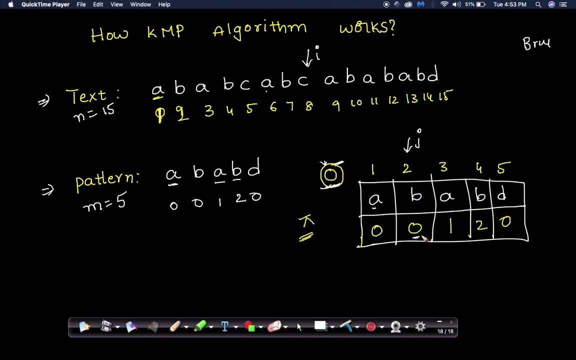 moving, moving my j pointer to this position. that is the zeroth position. okay, right now my j is pointing to the zeroth position. then i will repeat the same step. then what we have to do: j plus one index is a. the value presented, the j plus one index, is a and ith index value is c. there is a. 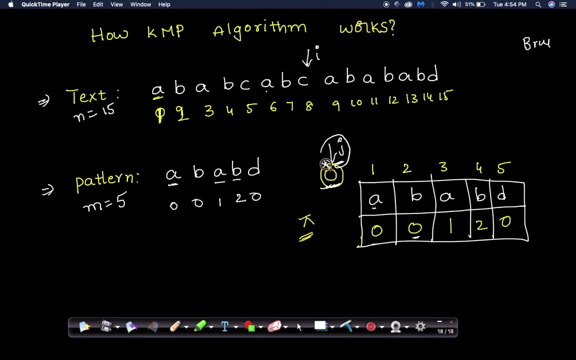 mismatch. then what we have to do- and right now i am at the starting position of j- then i'm going to increment the value of i by one. right now i am at the ninth position of the. i is pointing to the ninth position. okay, then i will repeat the same step. then i'm compare: j plus one index value is a. 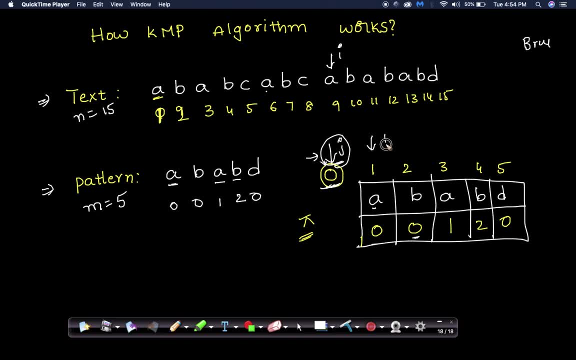 ninth index value is a. yes, it's a match. i'm going to increment the value of j by one and i'm going to increment the value of i by one. then i'm going to compare j plus one index value, that is b. yes, it's a match. then i'm going to increment the value of i by one and increment the value of j by one. 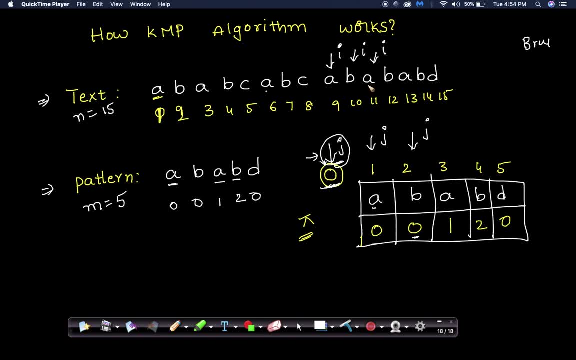 then j plus one index value is a and ith index value is a. yes, it's a match. then i'm going to increment the value of j and increment the value of i. right, then i again i'm going to compare j plus one index value, that is b, and ith index value is b. yes, it's a match. then what we have to do, we 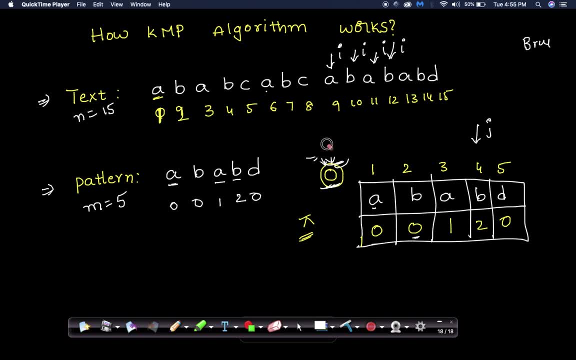 have to increment the value of j by one- okay, and increment the value of i by one- okay, and right now we have to move j plus one index value to j plus one index value. that is a okay. that is there is a mismatch. then what we have to do? then what we have to do, we have to go back this position. 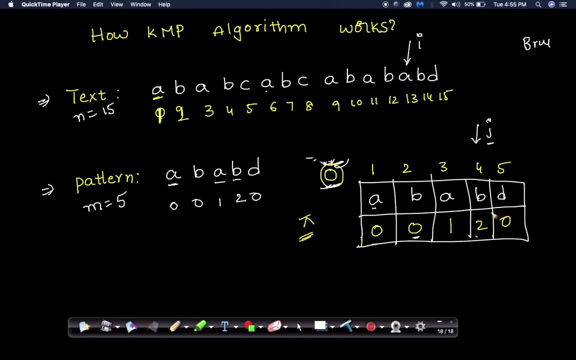 instead of moving back this i position to back here, i'm going to move my jth position according to this longest prefix suffix table. okay, according to this, we have to move my j pointer from fourth index to the second index. right now my j is pointing to the second index value. okay, then what? 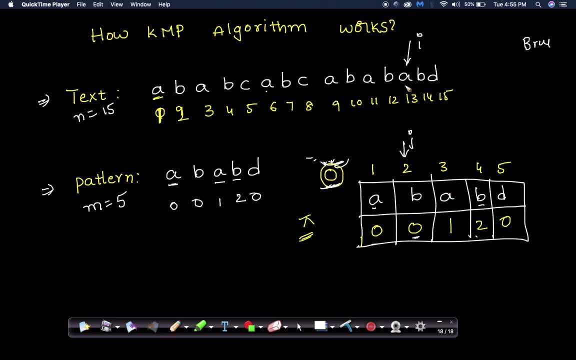 is a. i'm going to compare this ith value. that is a. yes, yes, it's a match, and what we have to do, we have to increment the, both the values. that is, j is pointing here and i is pointing to the 14th index. okay, and i'm going to compare: j plus one index value is b and i plus one index value is b. yes, 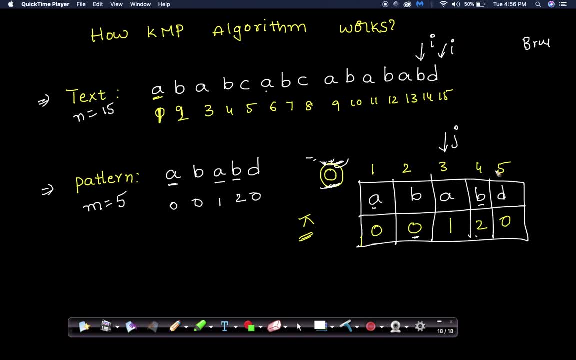 it's a match, then i'm going to increment the value of i by one and increment the value of j by one. i'm going to compare j plus one and i think x value, that is d, and d, yes, is a match. then we find the pattern at this position. okay, i hope you understand this right. 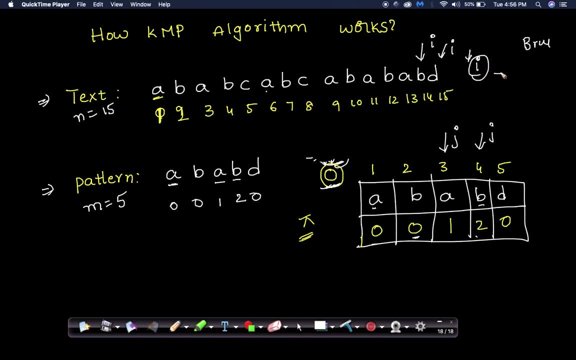 then increment the value of i and we have reached the end of the string. then we will stop the entire algorithm. i hope you understand this algorithm right. it's a very, very simple algorithm. once we able to construct this pi table or a longest prefix suffix table, okay then what is the time? 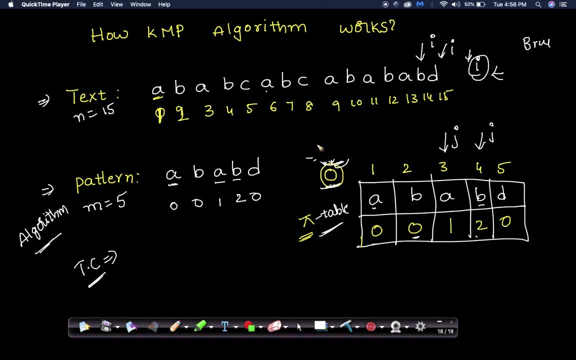 complexity of this approach. okay, according to this algorithm- and if you can notice here my i is traverse this entire input string only one time, right, only one time. that means how many characters are present in this entire input string, that is, n, number of characters, that is, and also we have 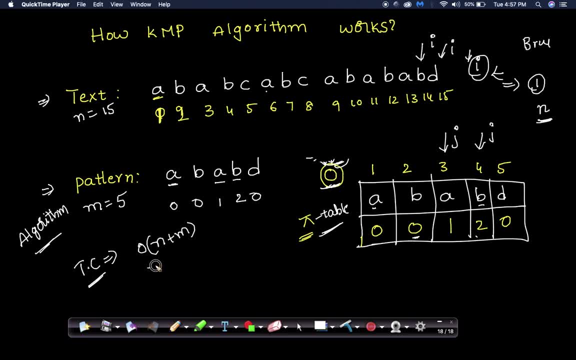 traverse this pattern, that is n plus m. i hope you understand this right then. overall time complexity of this problem is: this algorithm is order of n plus m. and what about the space complexity? we have constructed a pi table of size m. that is space complexity of this algorithm. 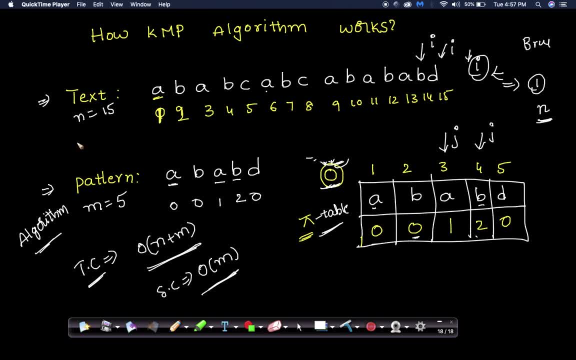 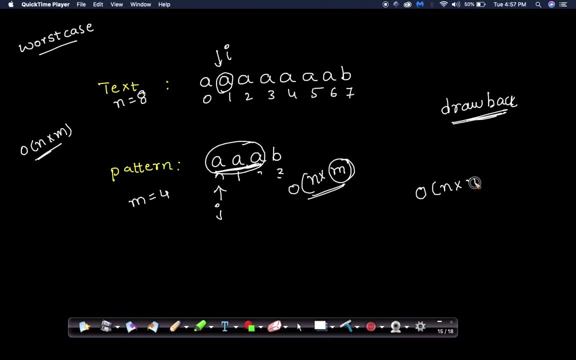 is order of m. okay, and this is the better algorithm than the brute force approach. right in the brute force approach, we have solved this problem in order of n into m. this is nothing but a quadratic time, and we have solved in a linear time, that is, m plus n time. okay, that is the basic. 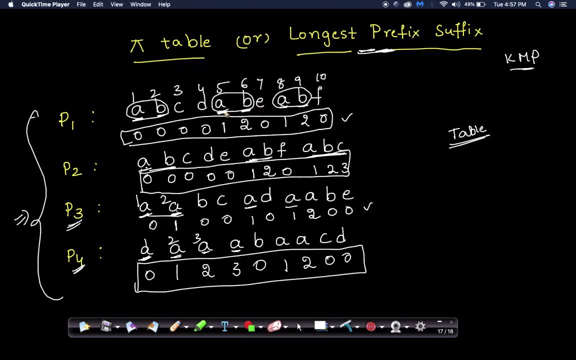 advantage of. that is, the beauty of the kmp algorithm is by constructing a pi table. okay, i hope you understand this right.